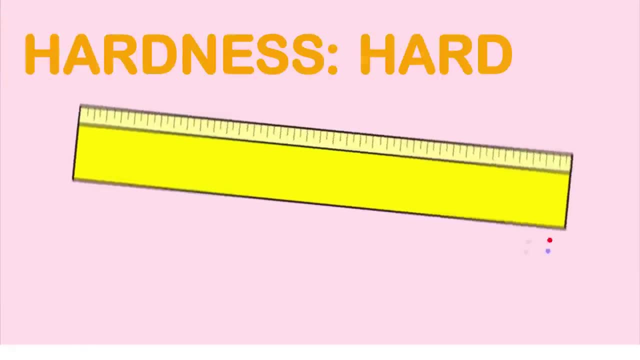 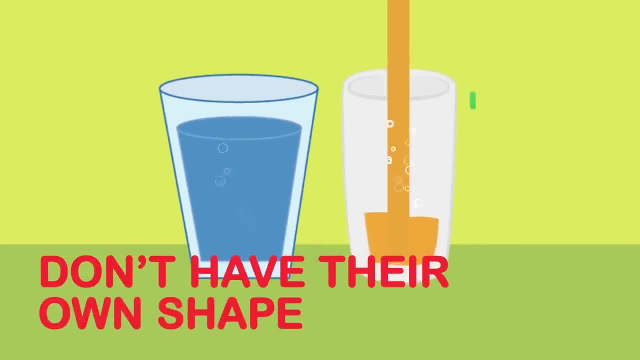 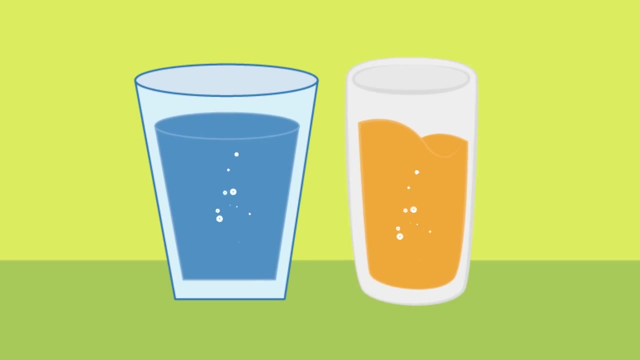 When you touch it, it's smooth. When you press it, it's hard. Liquid has color, smell and texture too, but they don't have their own shape. They always take the shape of whatever they're placed in, For example, slime. 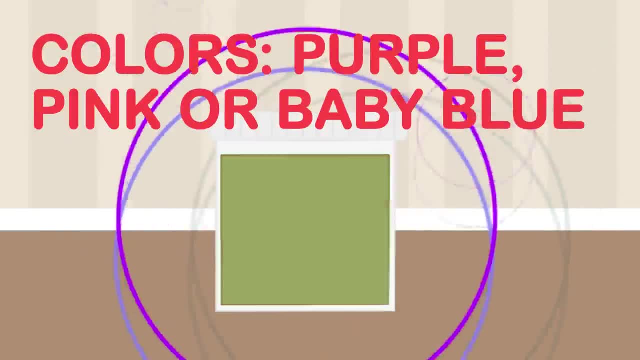 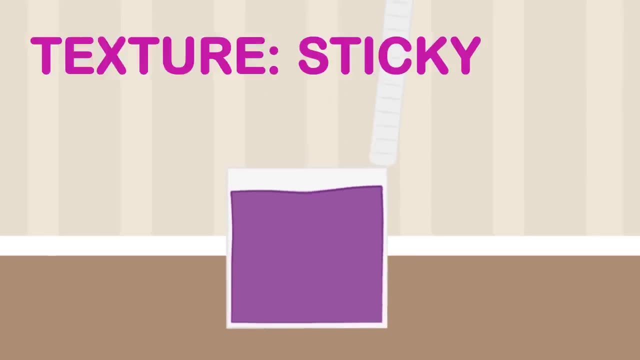 Everyone loves playing with slime. right? Slime can have different colors, like purple, pink or baby blue. They have smells. Some slimes smell different from other slimes. They also have texture. They're sticky, But they don't have their own shape. 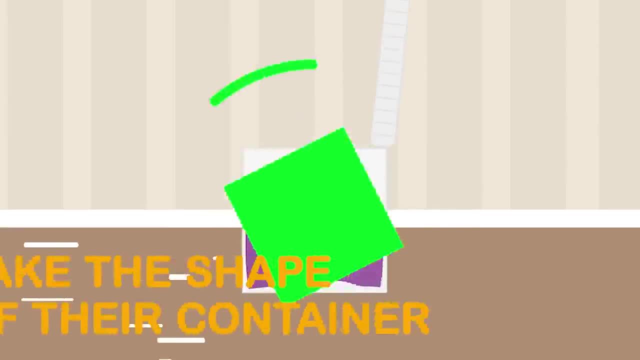 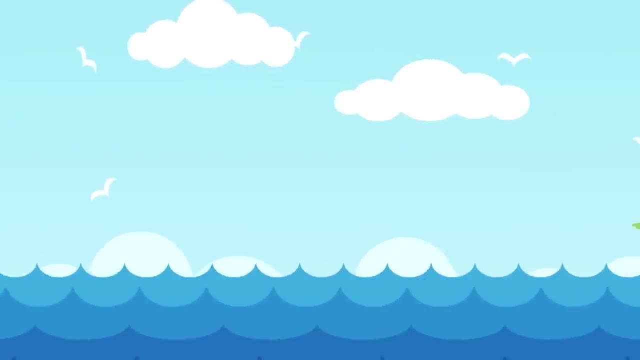 That's why, When you put them in a square container, they just fill the square, But when you take them out, they're not square right. Water is also a good example. When you go to the beach, you see all the seawater stretch before you. 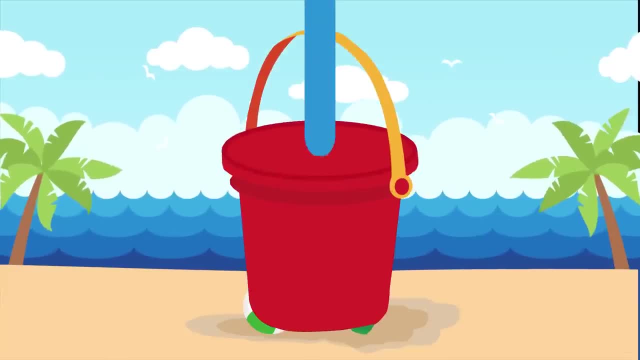 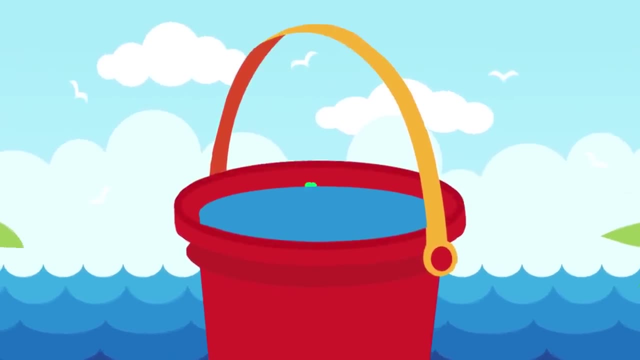 But when you take some seawater, for example, and put it in your sand bucket, it just fills the bucket and follows the bucket's shape. For example, if your bucket is shaped like a circle, the water is also shaped like a circle. 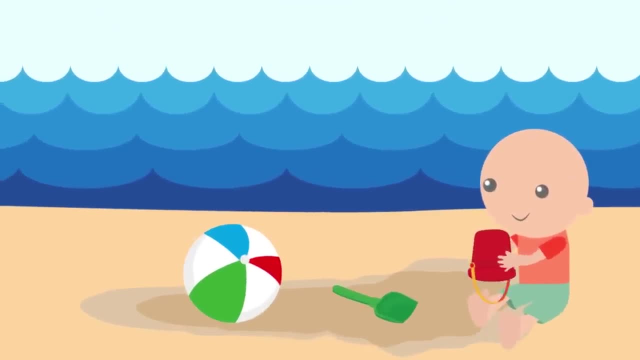 But then when you toss the seawater, you see all the seawater, And when you put the seawater on the sand, it's not a circle anymore. Gas, on the other hand, have no color, taste or texture. 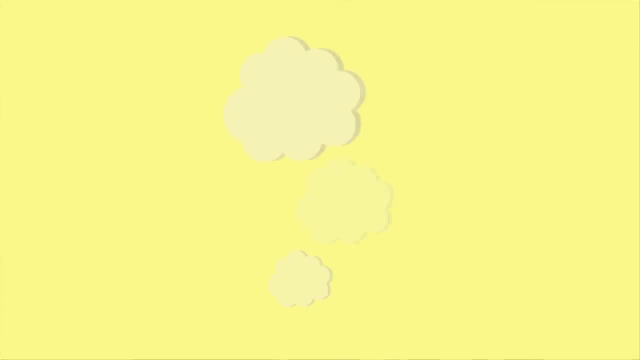 The rare times you do see them, they don't have their own colors, You can't taste them, and they don't have texture either, since you can't hold them in your hands. Like liquids, they have no definite shape and only take the shape of whatever they're put into. 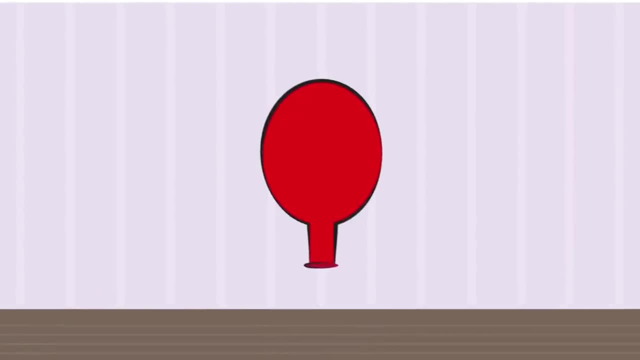 Let's take a balloon, for example. When you pump air- which is the gas- into the balloon, it grows into this big circular shape, Not because that's the shape of the air, But because it's the shape of the air. 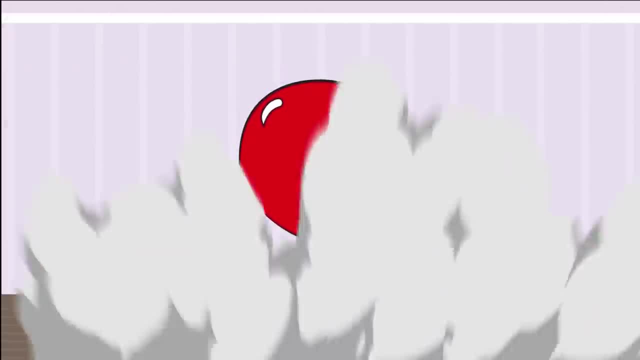 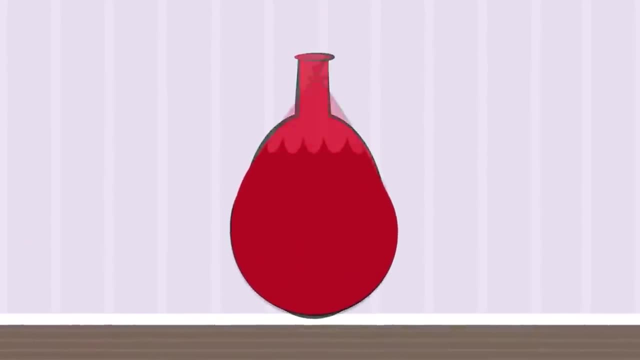 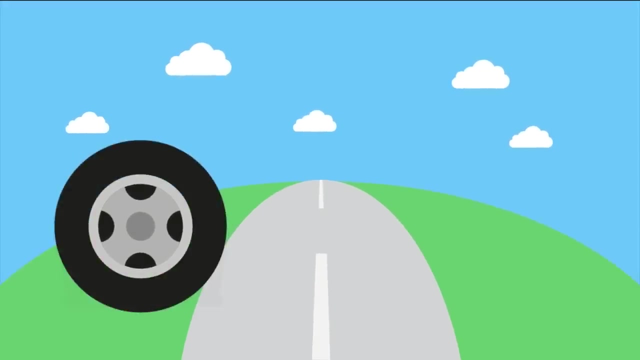 Not because that's the shape of the air, But because the balloon is expanding. When you put water into the balloon, since it doesn't have its own shape either, it is the same as the air-filled balloon. When you put air into a flat tire, you can see the tire being filled with air. 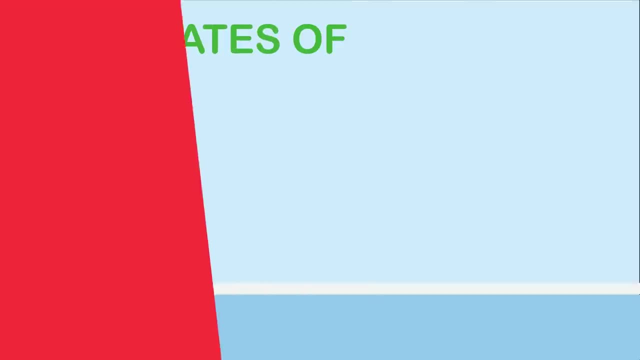 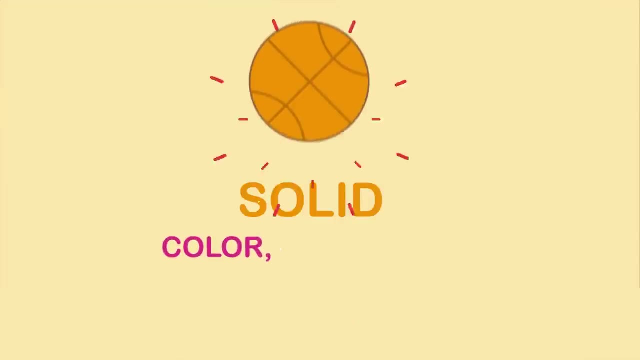 But the tire still has the same shape. Once again, the different states of matter- Solid, liquid and gas- have their own characteristics. Solid objects have color, size and texture, Shape, texture and hardness. Liquids have color, smell and texture.